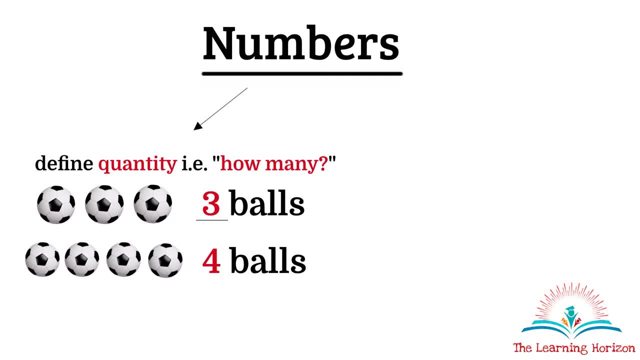 Same way. in this example, 4 is a number that tells me I have 4 balls. 3 and 4 are two different numbers. This shows 2 different quantities. Note: every number represents a different quantity. Numbers are sometimes used for labeling. 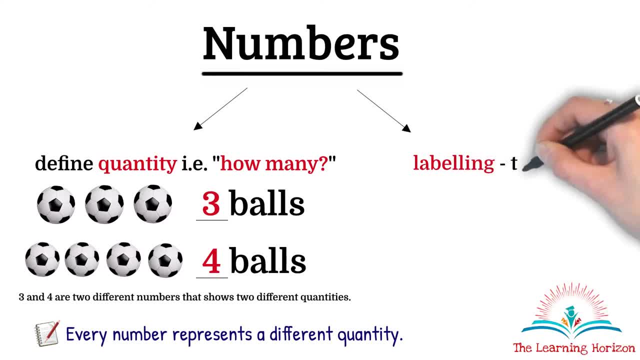 Labeling with numbers helps us identify and tell the things apart. Here we have 3 houses. They all look similar and identical, But I cannot tell them apart. So I can just say they look similar, them apart. i cannot identify them individually, but if i number them as 11, 12 and 13, i can. 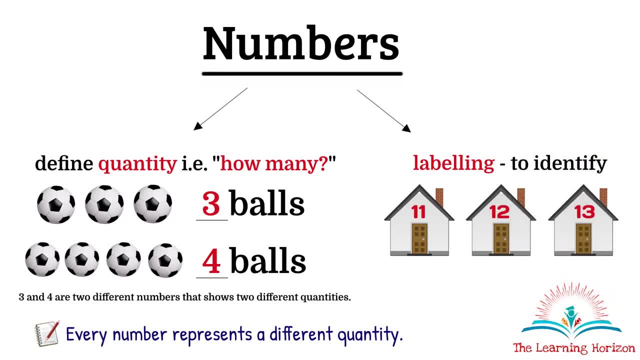 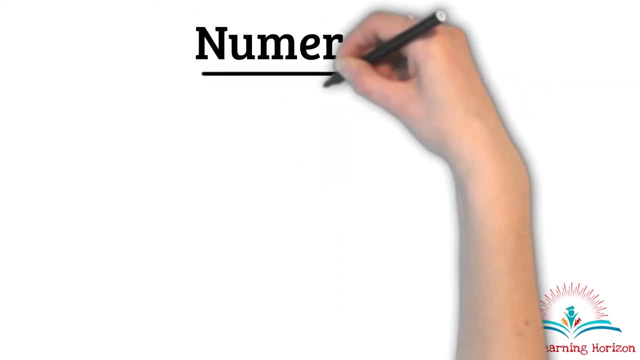 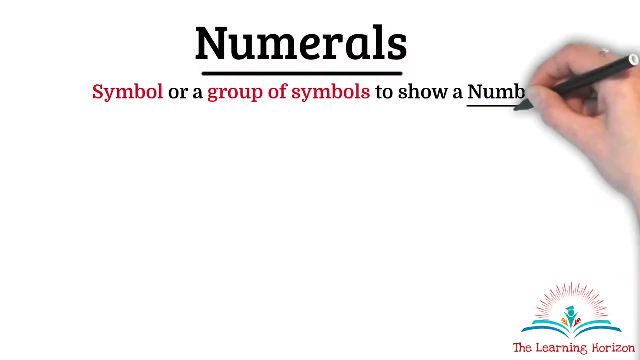 identify them. so, as we have seen with examples, numbers are used to define quantity and also sometimes used for labeling. now let us talk about numerals. numeral is a symbol or a group of symbols to show a number. let us take the same example to explain the concept of numerals. 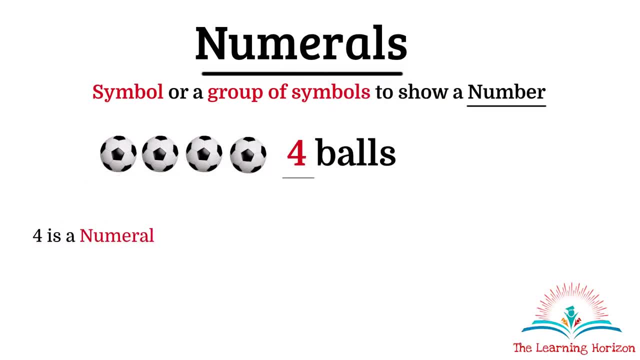 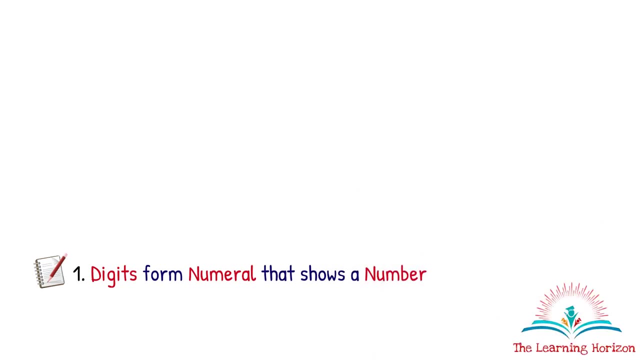 here four is a numeral. it is using digits, which is again a symbol, to show number 4. that is the quantity digits form numeral that shows a number. for example, here 4 is a single digit numeral to show a number 4. it has 1 digit, 4, 32 is a 2 digit numeral. 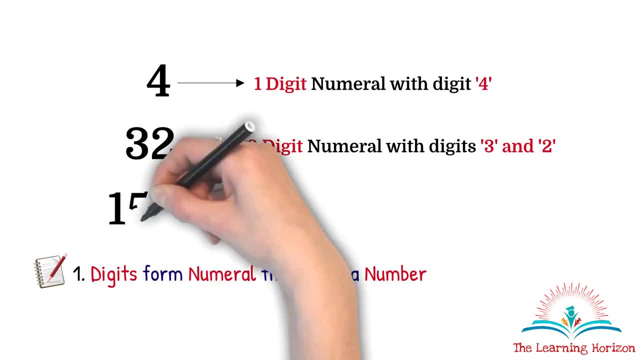 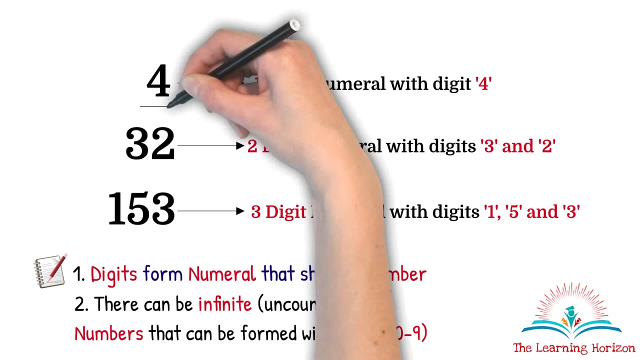 it has 2 digits: 3 and 2. 153 is a 3 digit numeral with 3 digits: 1, 5 and 3. there can be infinite numbers that can be formed with just these 10 digits. but is this the only way to show? 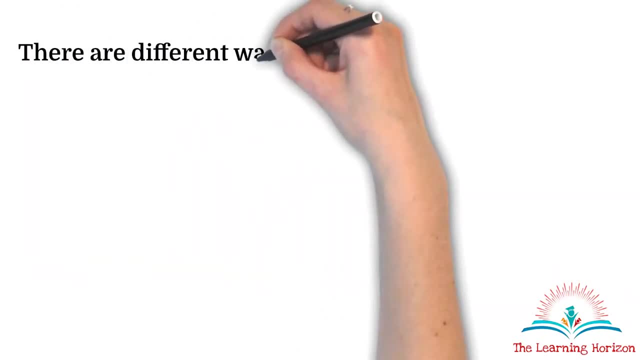 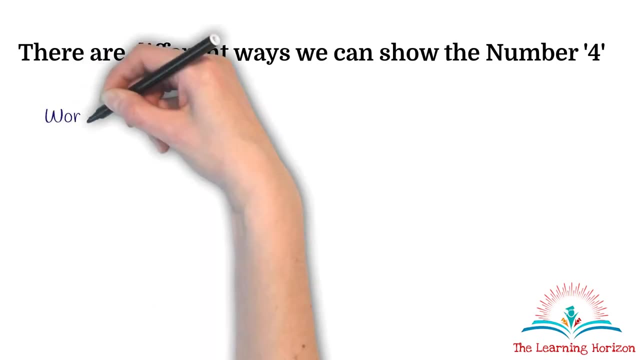 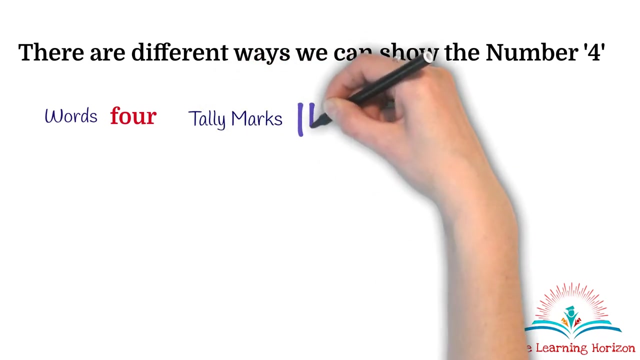 a number. no, there are different ways we can show the number 4, like i can write in words. i can write in words: that is f? o? u? r, it shows the number 4. or i can show using tally marks. that is 1, 2, 3. 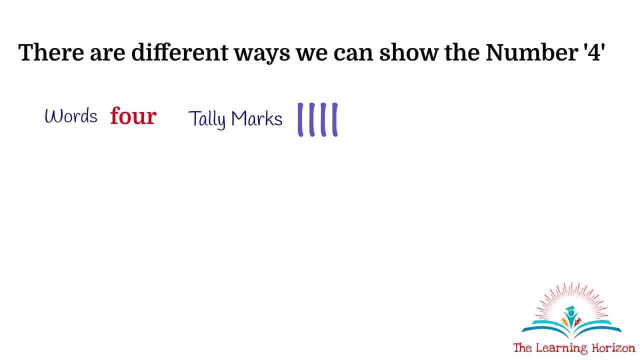 4. here i am using the tally symbols to show the number 4. i can also show the number 4 in terms of roman numerals. like i can use a 10 frame or a number line too. as you see, there are different ways you can show a number. 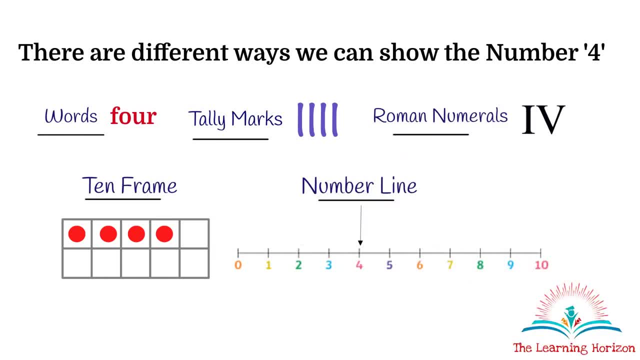 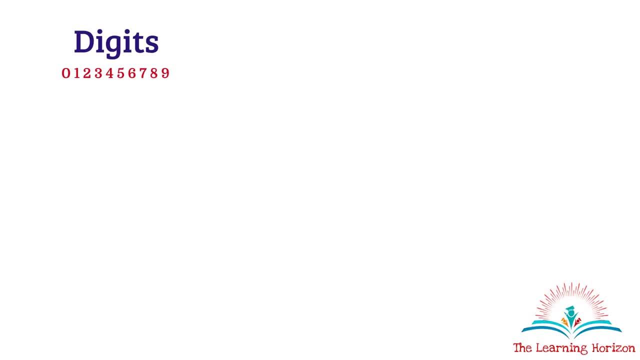 all these are different types of numerals showing the same number 4. so far we have learned that digits are 10 symbols. numeral is a symbol or group of symbols to show a number. numbers define quantity. let us quickly recap with an example. we will consider two digits, one, two. now we will group these digits to form two numerals, that is. 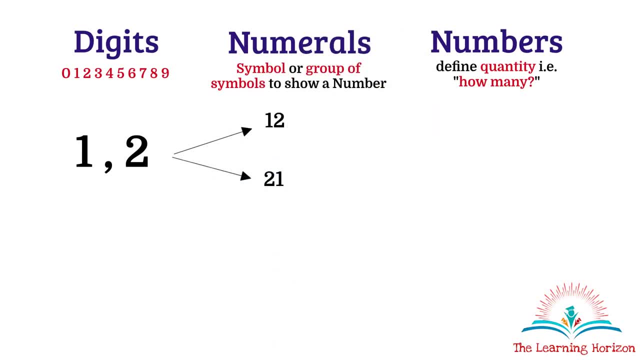 one, two, two, one. these numerals show a number that is quantity, and half, numberising the numbers pancake. this numeral here shows the number 12, that is a quantity of 12.. this numeral here shows the number 21, that is a quantity of 21.. 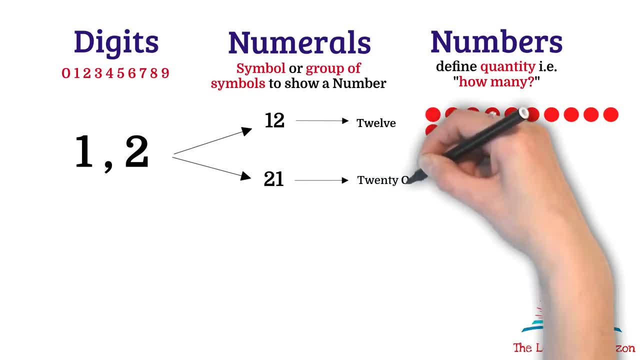 so now we have seen half digits to form numeral, to show a number. digits in math are like alphabets in english where we need to close one of two UM and one preview to get a Creativereich number ıl. the letters A to Z are different symbols. these symbols group together to form a. 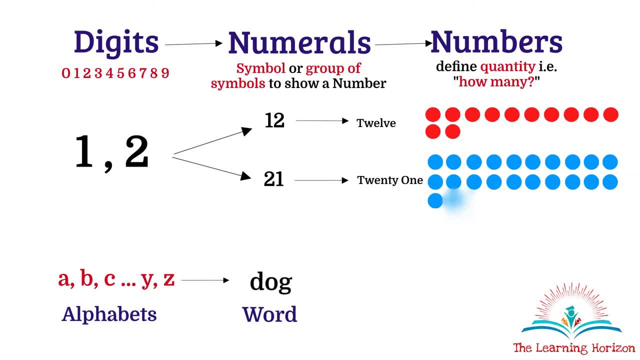 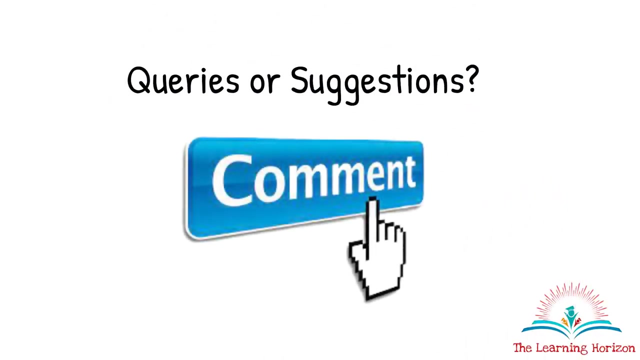 word which is like a numeral in math. this word stands for an idea and this idea is like numbers in math. hope this clears the basic understanding of digits, numbers and numerals. if you have any queries or suggestions, kindly leave a comment below. also, do not forget to check the description below for 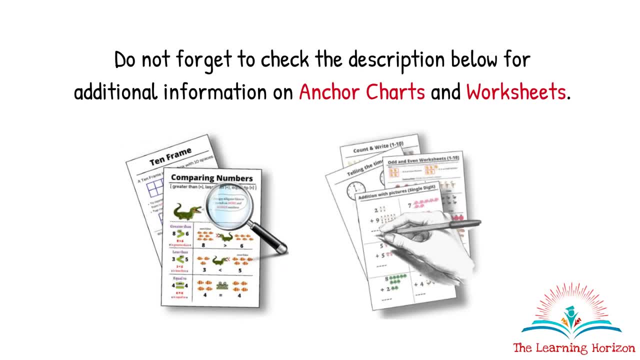 additional information on anchor charts and worksheets.